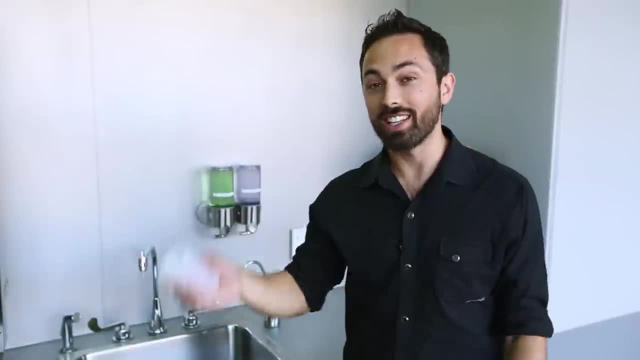 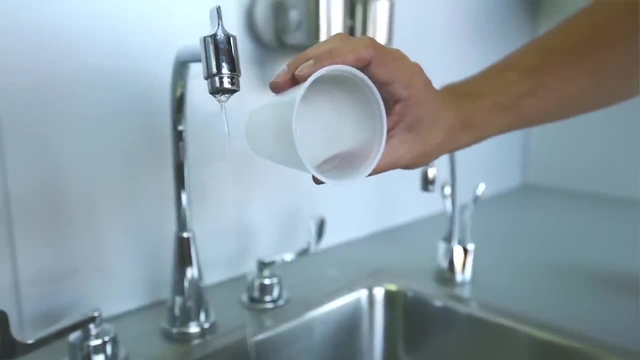 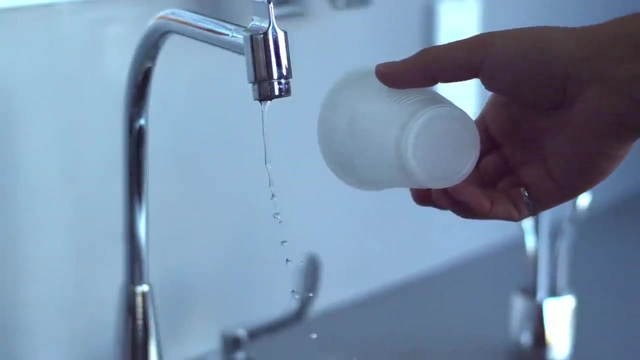 Why is it so? Number three: you've probably seen that if you rub a cup on your hair, you can make it electrically charged, and if you bring it close to a stream of water, you can actually cause that stream to deflect. Now, usually this is used in chemistry textbooks as a demonstration of the polar nature of 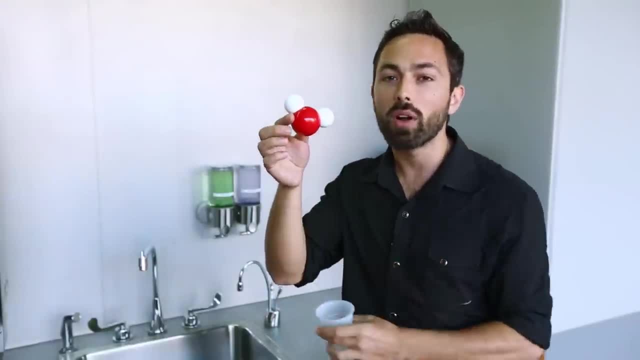 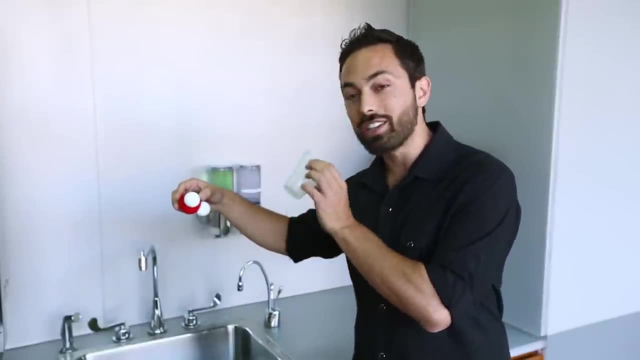 water. Water is a molecule with a more positive side and a more negative side, And so what happens, so you're told, is that the water molecule flips around, so the positive side of the water faces the negative side of the cup, and that is what attracts the water. 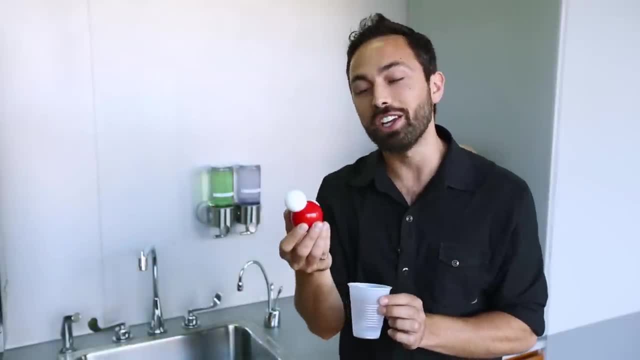 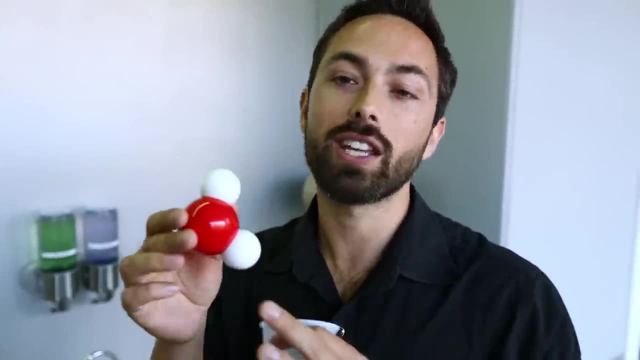 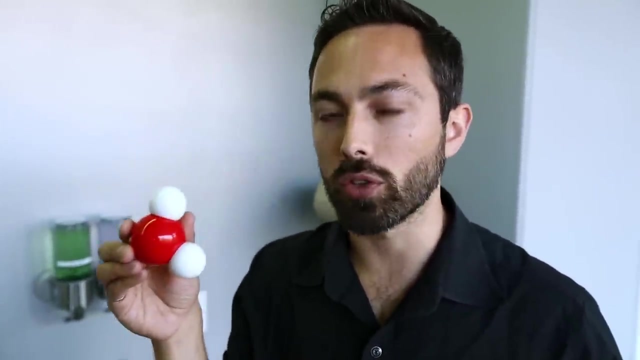 to the cup. But this is not the real explanation. Number four: If you have a uniform electric field, there's an equal force pulling the positive side towards it as there is pushing the negative side away from it, And so you can't actually do more than just turn the molecules. 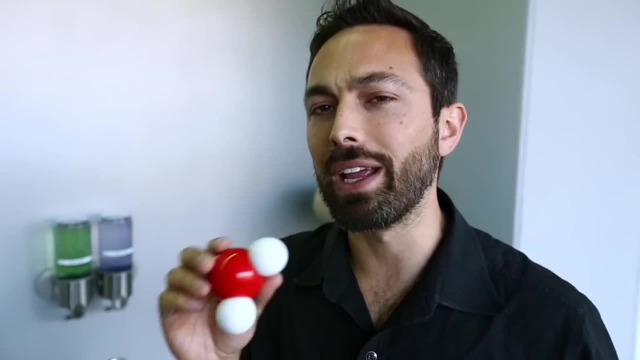 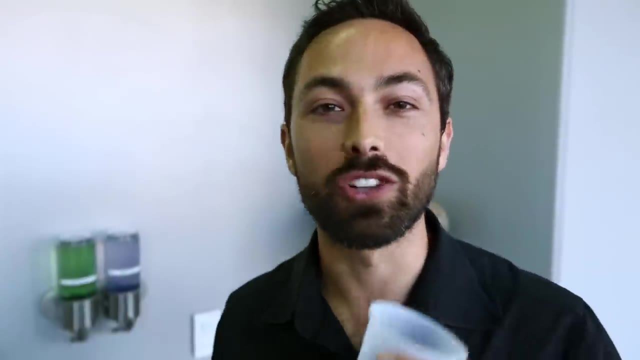 You would need a really, really strong gradient in your electric field to make this work at all, and it basically is just not going to happen from a cup. So why is the stream actually attracted to a charged cup? That is the question Number four. 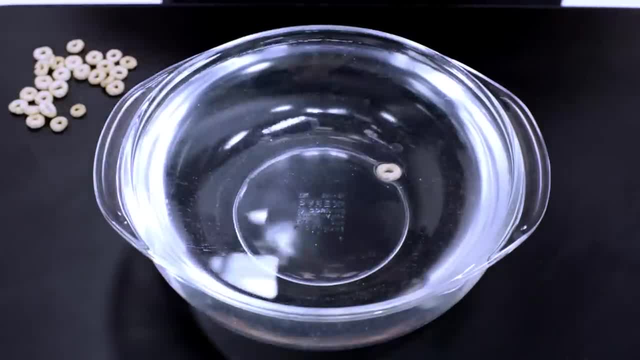 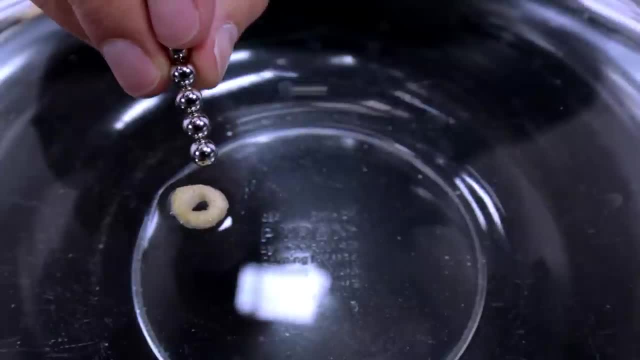 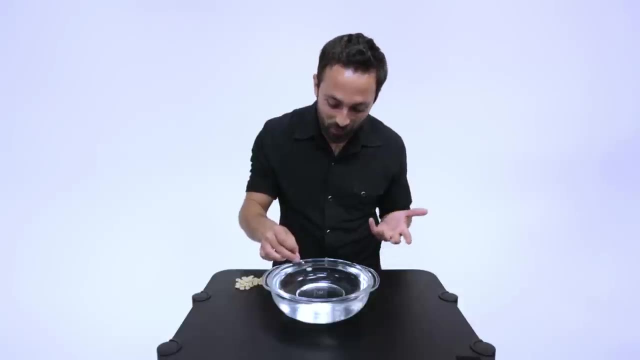 Take a piece of your favorite cereal and drop it into a bowl of water. Then, using a very strong magnet, try to pull the cereal around. Isn't that cool? So why is cereal magnetic? And finally five, The teabag rocket. 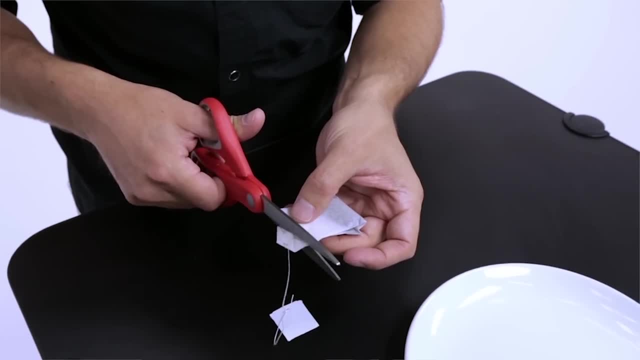 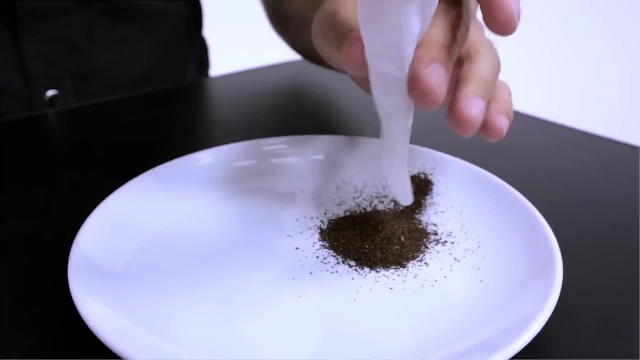 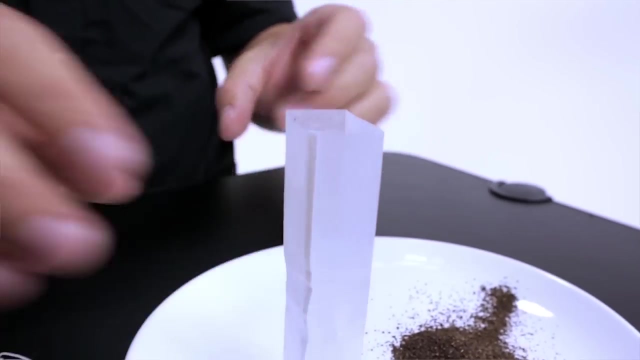 Take a teabag and cut off the sealed end very carefully. Now. Now Let's cook the tea. Form the teabag into a square column and balance it on the plate. Now, light the top of the teabag on fire. 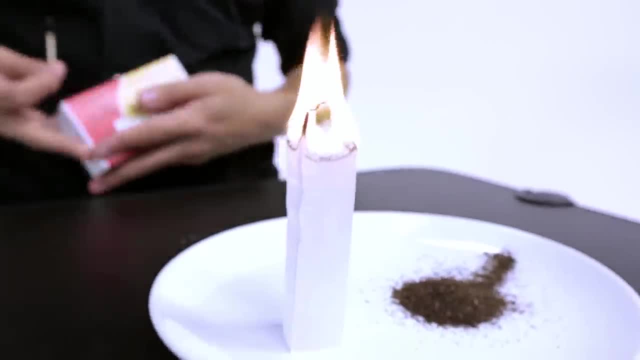 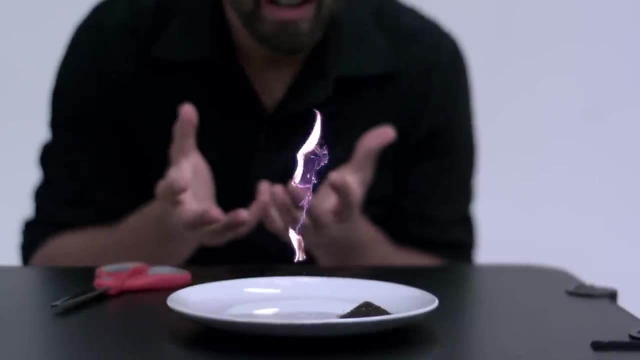 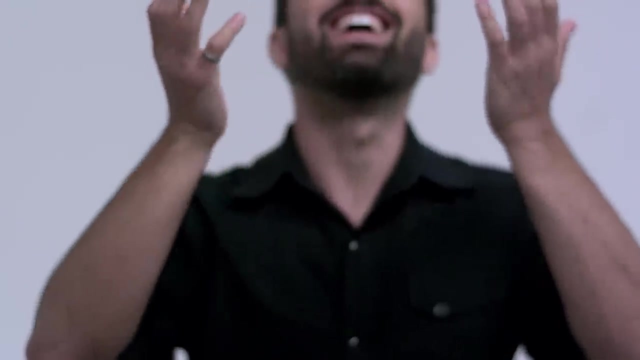 Try to light it evenly on all sides. Get ready for take off In three, two, one, Ha Yeah, That is the beauty of the teabag rocket. So why did that happen? So how do all of these phenomena work?